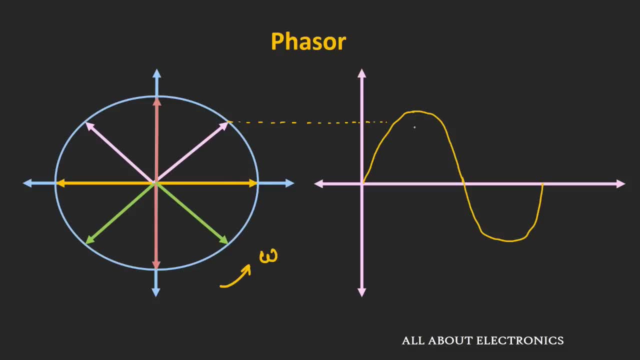 sinusoidal signal. So now let's see how we can represent this phasor on a phasor diagram. So now, on this phasor diagram, different AC sinusoidal signals, which is, having a same frequency but different amplitude and different phase, are represented. 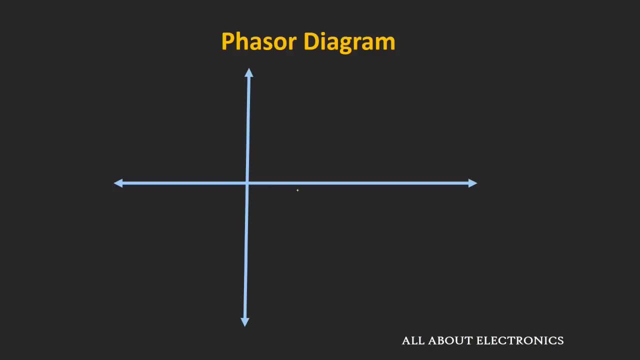 So while representing these phasors on this phaser diagram, we only represent them by amplitude and initial phase. So let's say we have two sinusoidal signals. Since we have two sinusoidal signals, I have to compute, let's say, its amplitude, with this. 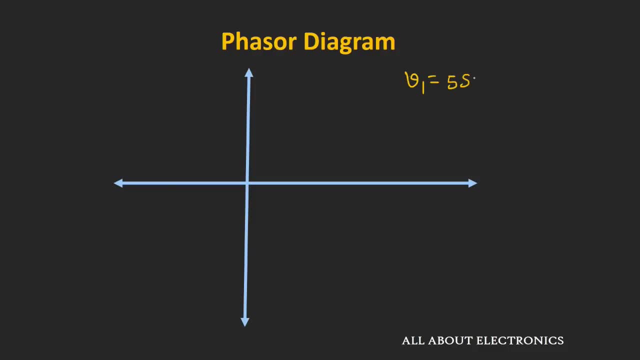 initial phase sinusoidal signals. the first is, let's say, 5 sin and the second signal is V2 is equal to tan and we want to represent these two signals in terms of the phasors in a phasor diagram. So the first signal is 5 sin. So first we will draw. 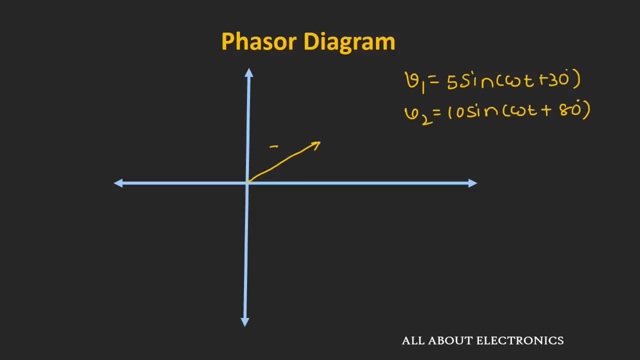 the vector, which is having an amplitude of 5, and it will make an angle of 30 degree with the horizontal axis, or a reference axis. Now, if you see the second signal, that is tan sin. So here the peak amplitude of this signal is tan. So we will draw a vector. 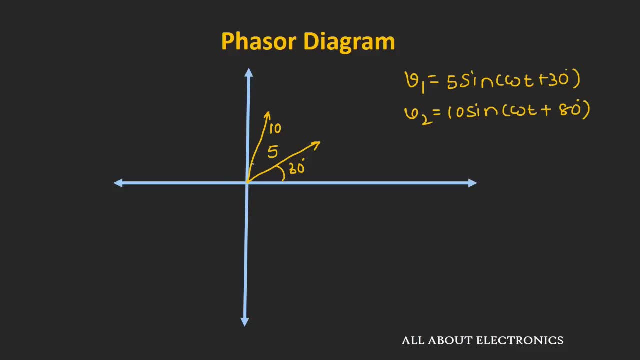 which is having a magnitude of tan, and it will make an angle of 80 degree with the horizontal axis. Now, sometimes this phasor is always in the phasor diagram, So this is also represented by the RMS value of the sinusoidal signal. 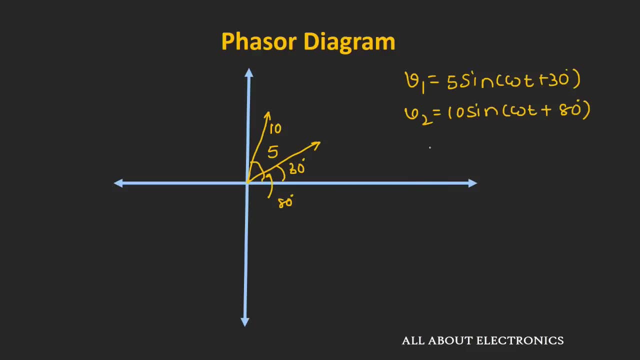 The reason is that most of the measurement which is being carried out by the ammeter and the voltmeter are in terms of the RMS values. So sometimes you will find that these phasors are represented by the RMS values instead of the peak value, But in this video 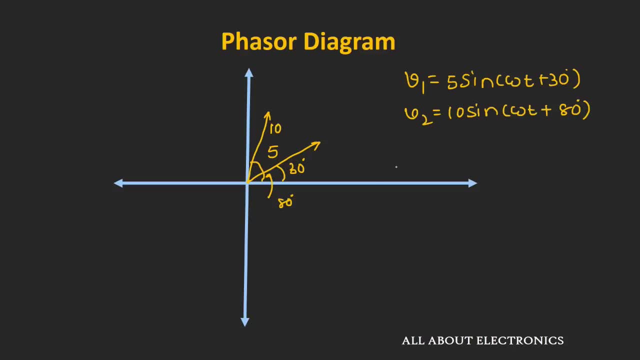 we will consider the peak values of these sinusoidal signals. So now let's see one more example based on this phasor diagram representation. So let us say, now we have a voltage That is equal to tan sin, and the second voltage, or second signal, is: 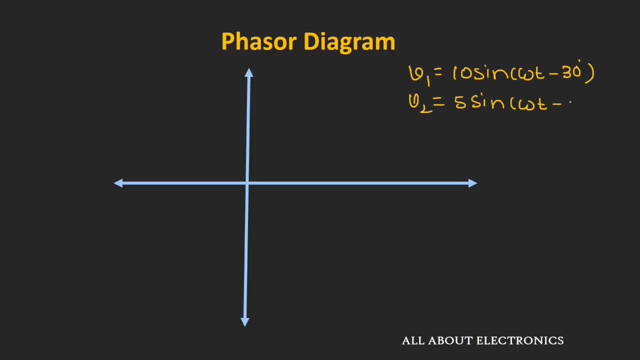 5 sin, And we want to represent those signals on this phasor diagram. So the first signal is tan sin. So we will draw a vector which is having an amplitude of tan And it will make an angle of minus 30 degree. So we will draw a vector. 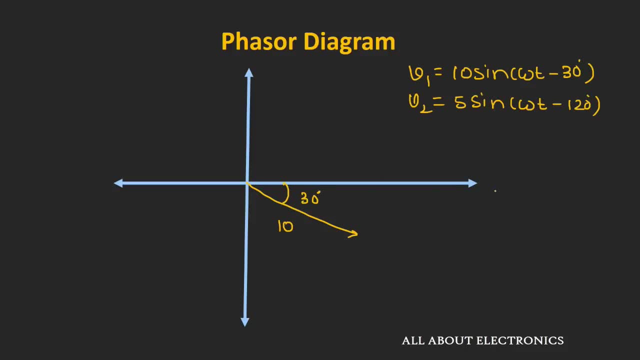 which is having an amplitude of 10, and it will make an angle of minus 30 degree, So 30 degree with the horizontal axis. Now, second, we will draw the second signal, which is having an amplitude of 5, and it will make an angle of 120 degree with this horizontal. 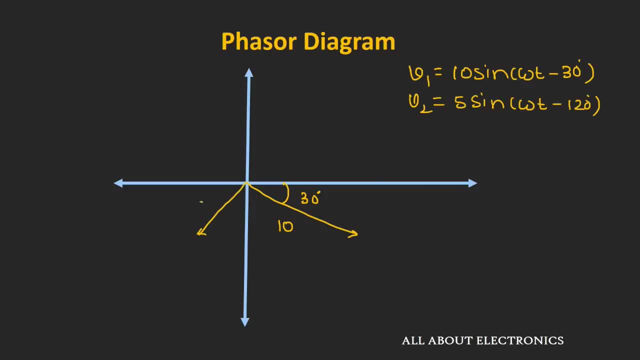 axis, So we can draw a vector of 5 amplitude and having a phase shift of 120 degree. So this will be the representation of V2 and this will be the representation of V1.. Now on this phasor diagram, this anticlockwise. 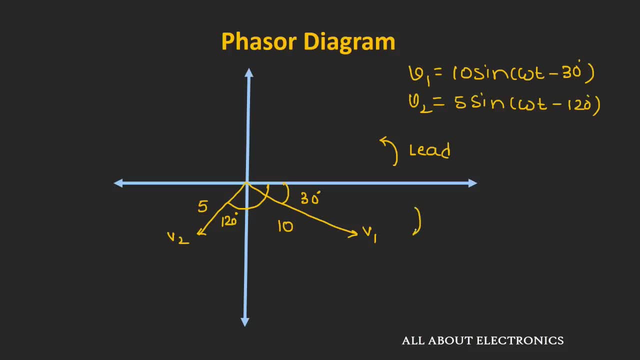 direction is known as the leading direction and this clockwise direction is known as the lagging direction. So, as you can see, here this V1 is leading the V2 by 120-30, that is, by 90 degree. So here this V1 signal is leading the V2. 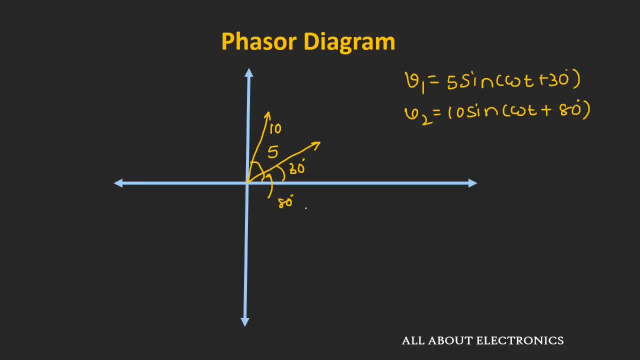 by 90 degree. Similarly, in the first case, if you see, this V2 signal is leading the V1 signal by 80-30, that is, by 90 degree, That is, by 50 degree. So now, so far we have seen that how to represent. 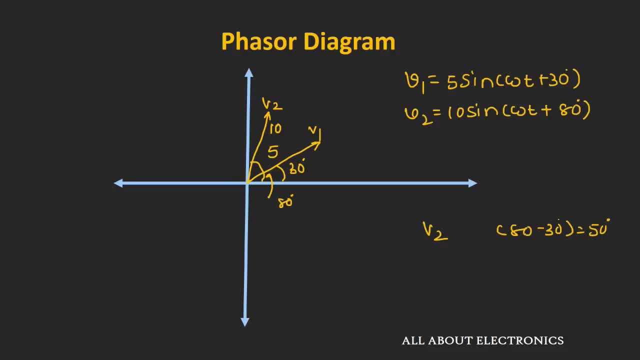 the phasor on a phasor diagram. Now let's see how we can represent this phasor in a mathematical form. So the first form is the polar form, where we can represent this phasor in terms of Rnθ. So suppose we have a phasor which is having 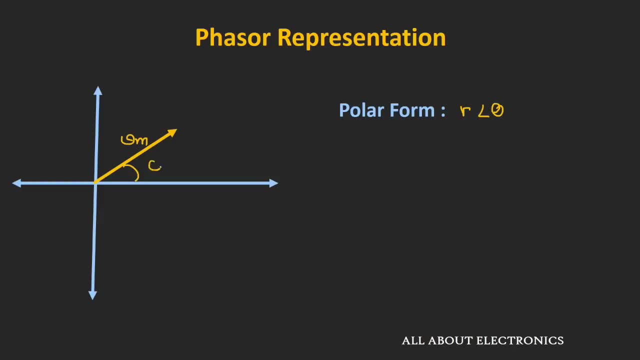 an amplitude of Vm and it makes an angle of 5 with the horizontal axis. then in the polar form we can represent it as Vm and 5.. So the next form is the rectangular form. So in this form we can represent any phasor by a complex number, that is, a plus jb. 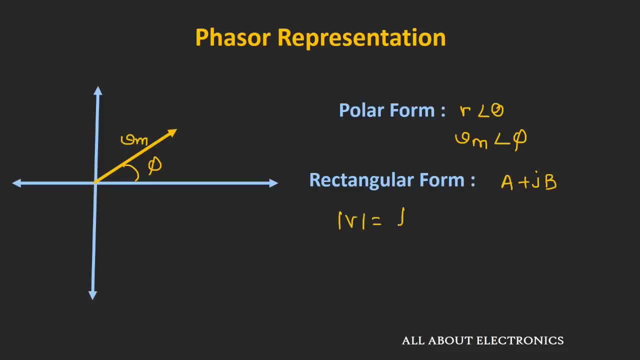 So the amplitude of this phasor will be under root and the phase of this phasor can be given by the expression tan-b by a. So this will be the rectangular form of representation of this phasor. Now the third form of representation is the exponential form, where we can represent the 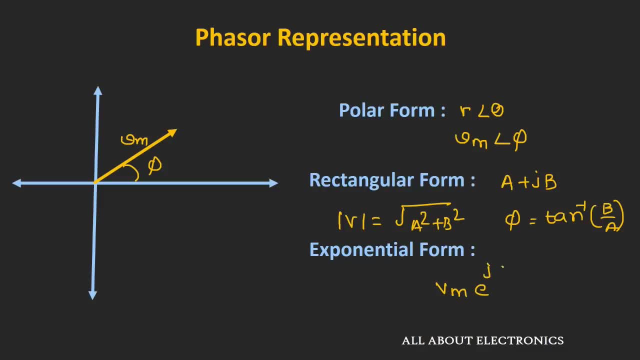 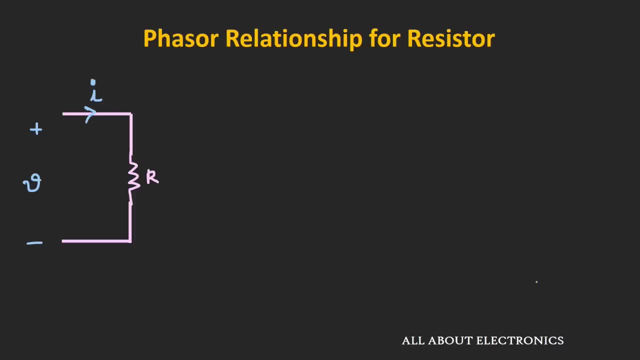 phasor in terms of Vm-t to e, to the power of j5.. So these are the basic three representations by which we can represent this phasor. So now, as we have seen how to represent any phasor in a phasor diagram as well as by a mathematical expression, 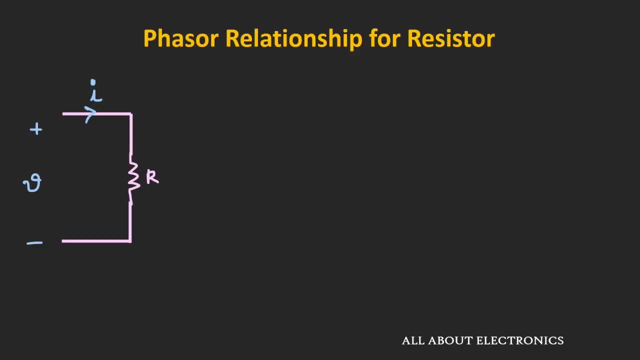 Now let's see the phasor relationship between the voltage and current for the basic circuit elements like resistor, capacitor and the inductor. So first we will see that the phasor relationship between the voltage and current for the resistor. Now let's say we have applied this sinusoidal input to this resistor. 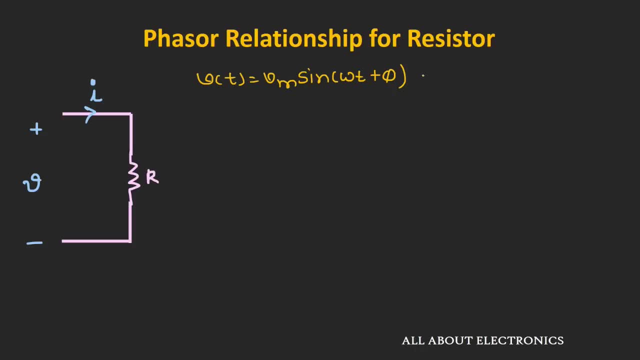 So this voltage signal can be represented in a phasor form as Vm x 5, where Vm is the peak amplitude and 5 is the initial phase. Or simply we can say that this is nothing but capital V. Now, according to Ohm's law, the current 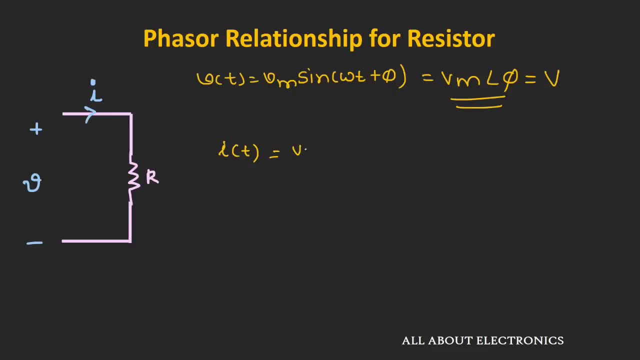 IT that is flowing through this resistor will be Vm, x sine ωt plus 5 divided by R. And if we write this equation in terms of the phasor form, then we can write it as I: that is equal to capital V divided by R, where here I and V both are in the phasor form. 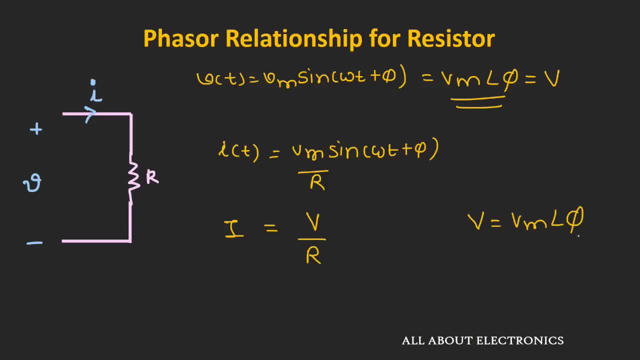 That means V is nothing but Vm over 5.. So now, as you can see here, both the voltage and current are in a phase. So if we represent this voltage and current on a phasor diagram, then it will look like this: 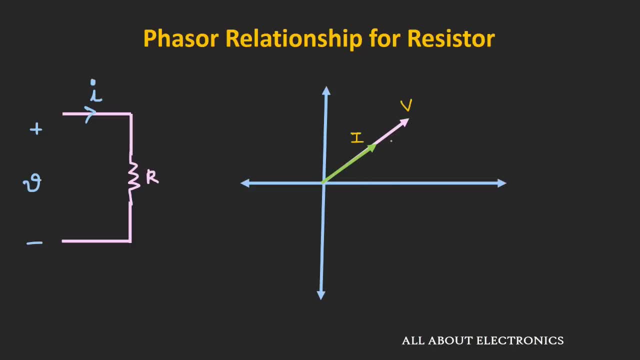 So, as you can see, here both the voltage and current are in a phase. Now, here the ratio of the voltage over current is 0.. is also known as the impedance. So for the purely resistive circuit the impedance is equal to the resistance. Similarly, now let's see the phasor relationship. 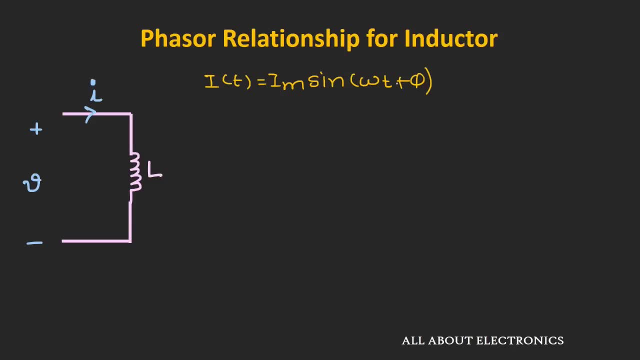 between the voltage and current in the case of inductor. So now let's assume that the current that is flowing through this inductor is given by this expression, that is, Im sin, Or, in terms of the phasor relationship, we can write it as Im x- 5 or simply capital I. Now we know that the inductor voltage can 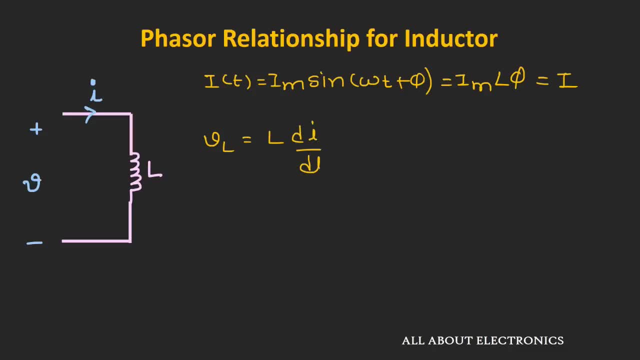 be given by the expression L× di × dt, Or you can write it as Ω× prim cos, Or we can write it as ΩL×Im sin. So this leads the current by a 90 degree. So, in terms of the phasor relationship, if we see then, 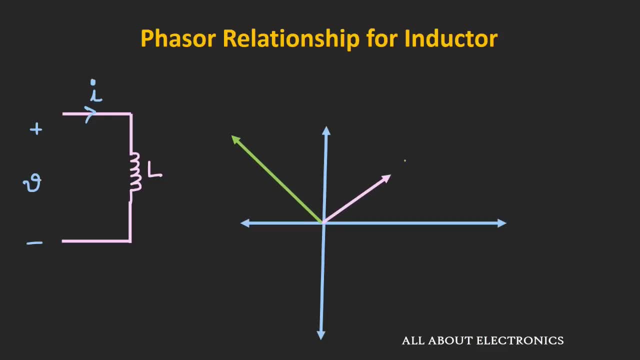 the phasor diagram will look like this. So here is the current that is flowing through this inductor, and the voltage will lead the current by a 90 degree. Now suppose if we represent this signal in terms of the phasor, then we can write it as ωl into e to the 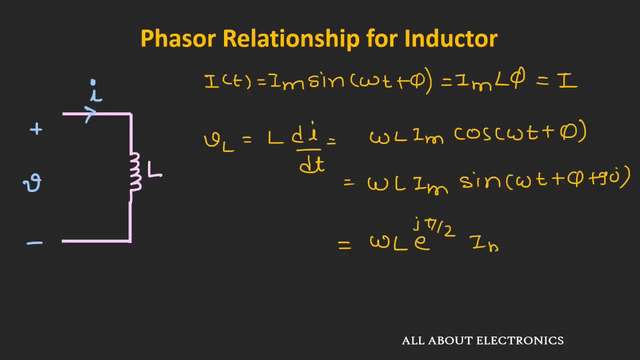 power of jπ by 2 into Im, into Φ, And we know that e to the power, jπ by 2 is nothing but j, So we can write it as j into ωl, into just I, where I is nothing but Im into. 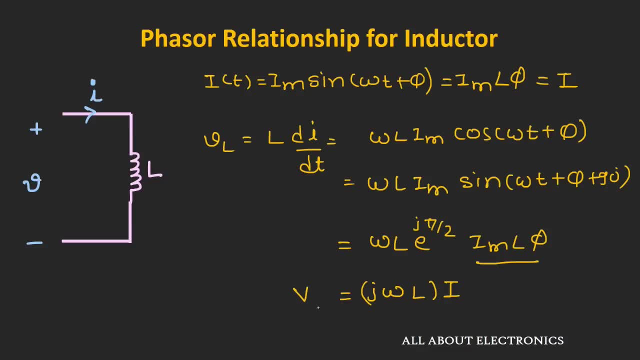 Φ. So this will be the expression for the voltage across the inductor in terms of the phasor form. So now we know that the ratio of voltage over current is nothing but the impedance. So here we have seen that this voltage can be given by the expression j into: 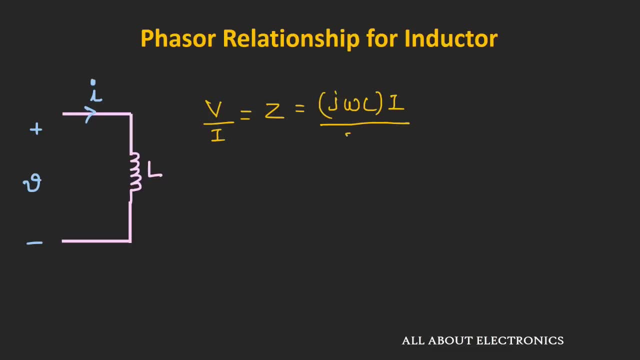 ωl into I, And here both capital V and capital I are the voltage and current across this inductor in terms of the phasor form. So we will get the impedance Z as j into ωl. So we can say that for the 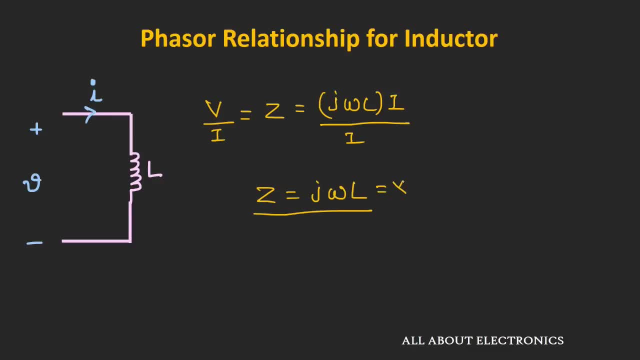 purely inductive circuit, the impedance, or simply a reactance of this inductor will be j into ωl. So now, similarly, let's see the phasor relationship for the case of a capacitor. So here let's once again assume that the capacitor voltage that is applied to this 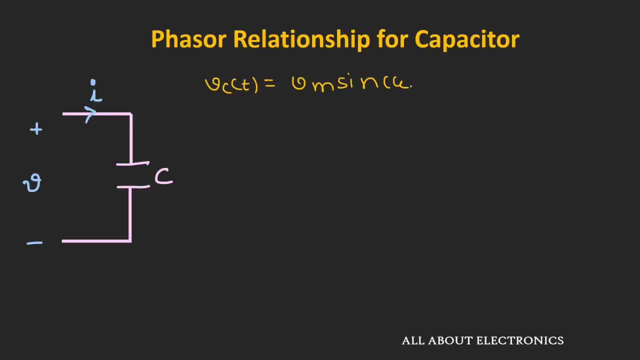 capacitor is Vm into sin, ωt plus 5.. We know that the capacitor, current Ic, can be given by the expression C into dV, by dt, that is, C into ω, into Vm, cos of ωt plus 5, that is nothing but ω, C into Vm, into sin. 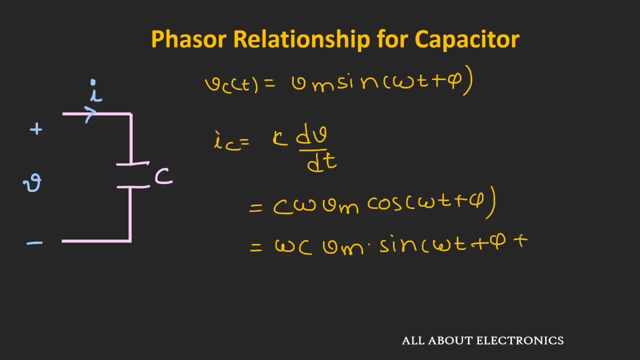 of ωt plus 5.. So this will be the expression for the current that is flowing through this capacitor And, as you can see here, the capacitor current leads the voltage signal by a 90 degree. So in terms of the phasor representation, if you see, it will look like this: 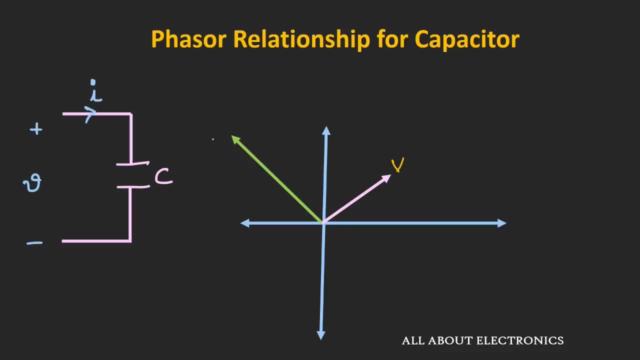 So if this phasor represents the voltage, then the current will lead the voltage by a 90 degree. Now suppose if we represent this signal in terms of the phasor form, then we can write it as: I, that is equal to ωc, e to the power of jπ by 2, into Vm, into 5.. 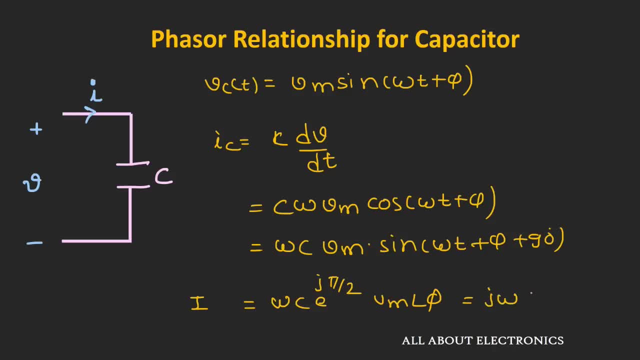 Or we can say that J into ωc, into V, where V is nothing but Vm into 5.. So this expression is nothing but the current that is flowing through this capacitor in a phasor form And, as we have seen earlier, the ratio of voltage, current and voltage is nothing but. 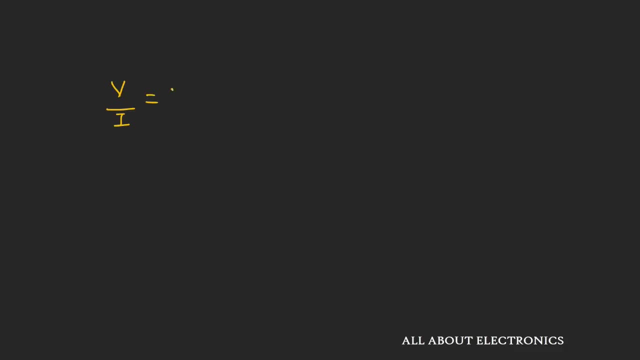 Vm into 5.. So, as we have seen earlier, the ratio of voltage is nothing but Vm into 5.. voltage over current is nothing but the impedance And here, as you can see, it is nothing but 1 over j into ωc. So we can say that for the purely capacitive circuit, the impedance, 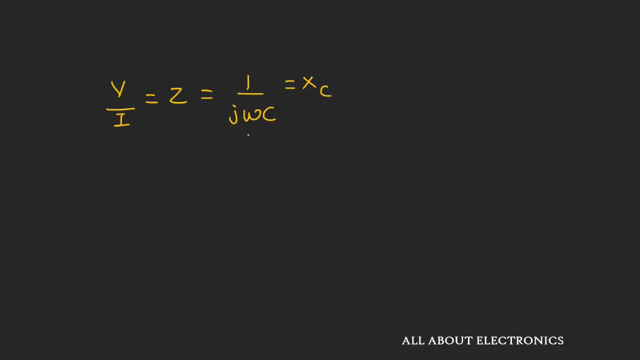 or simply reactance of the circuit will be 1 over jωc. So in a summary, we can say that for the resistive circuit, the current and voltage will be in a phase, While in case of a purely inductive circuit, the voltage will lead the. 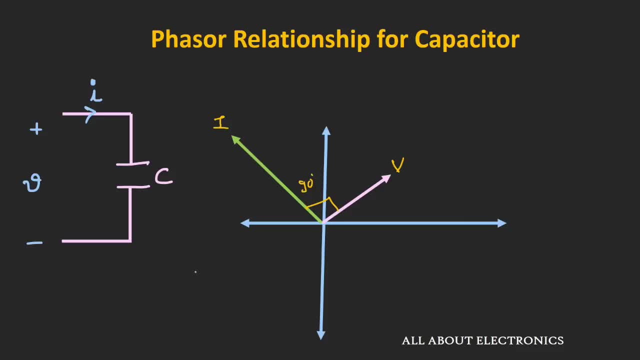 current by a 90 degree And in case of a purely capacitive circuit, the current will lead the voltage by a 90 degree. So now suppose if we want to remember this voltage and current relationship across this resistor, capacitor and inductor, then we can remember this just. 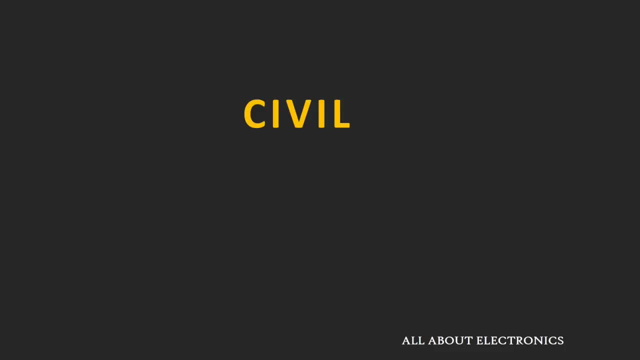 by using this simple keyword, that is a civil. Now, if you see this word, if you see the first three letters, that is Ci and V. So we can say that in capacitor the current leads the voltage by a 90 degree. 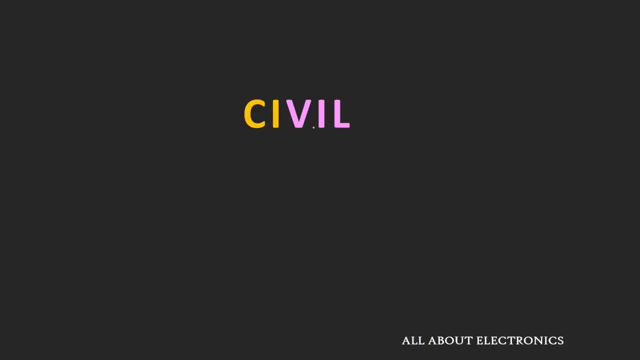 And if you see the last three words, that is, Vi and L, then we can say that in inductor the voltage leads the current by a 90 degree. So in this way we can remember that in case of capacitor the current leads the voltage And in case of an inductor the voltage leads. 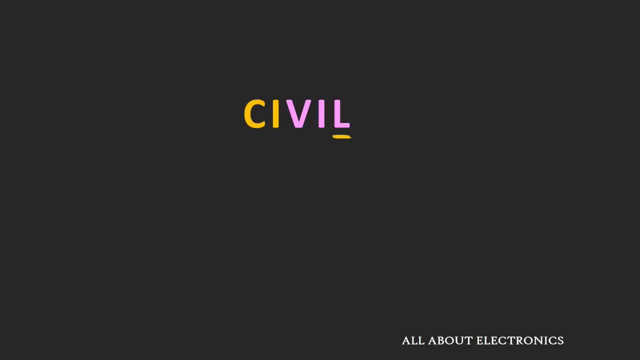 the current by a 90 degree. So now in the next video we will see that- how to draw the phasor diagram for the RL RC as well as the RLC circuit, And we will also solve some problems related to these phasors.